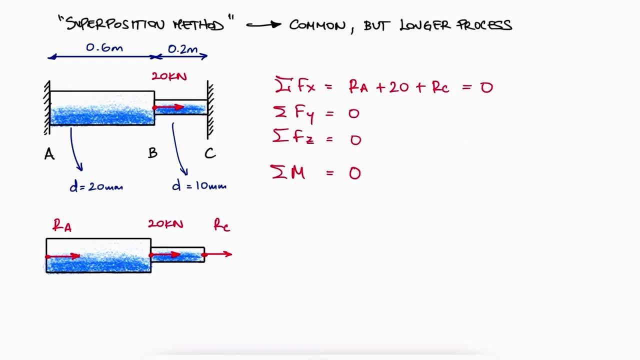 equations. None of the three sum of forces equations, nor the sum of moments, equations about any location within the structure, will give us enough information to solve for the unknown variables. In this case we use the axial deformation expression we developed in the previous lecture to add one more equation that will give us the missing information. 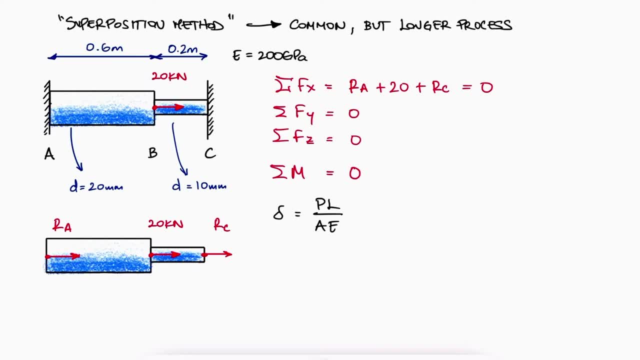 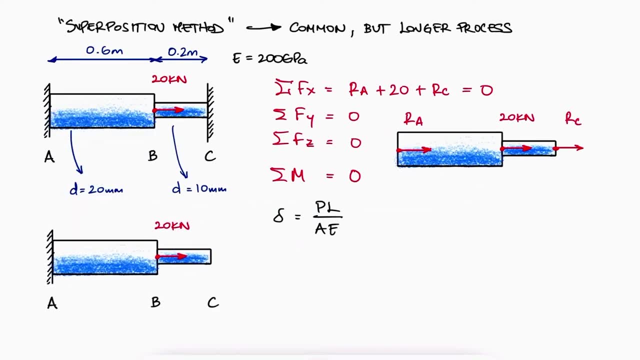 To briefly explain this superposition method I mentioned earlier, in case your instructor does use it and requires it for the solution of your exams. we'll use this same example If, using the superposition method, we would remove one of the constraints and see how the structure deforms, For example, without the wall at C. 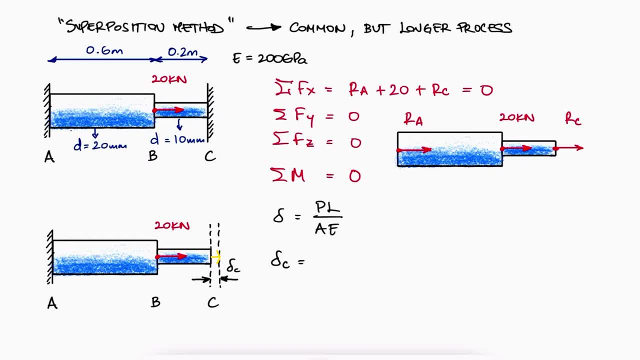 we could calculate the sum of forces in the X direction. by using the superposition method, We can calculate how much ABC is stretching, or its equivalent, how much C is being displaced now that there is no wall there. The displacement at C would be equal to that of B with respect to A. 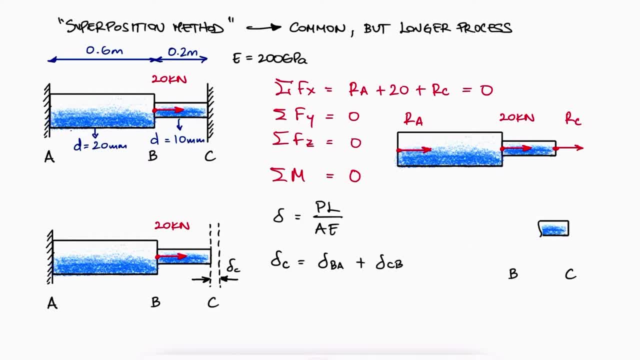 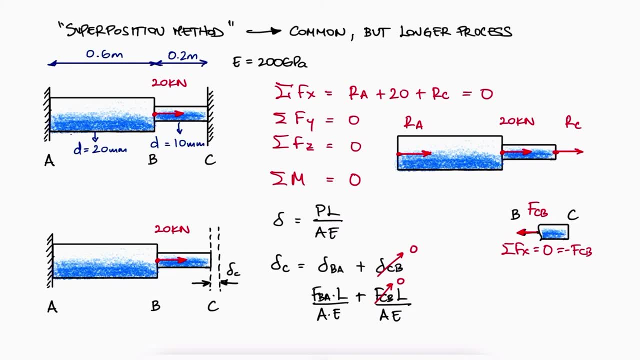 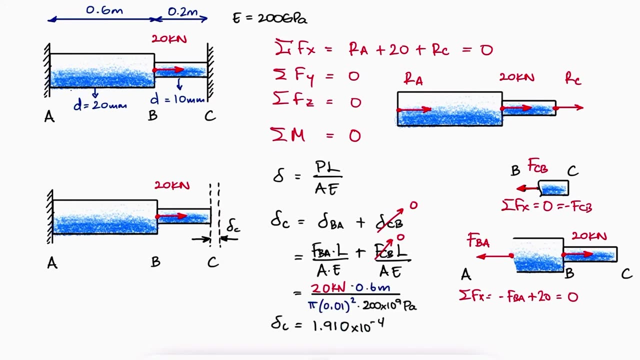 plus that of C with respect to B. Since there is no internal force between B and C, that deformation would be zero, and for B with respect to A, we would have an internal tensile force equal to the external load. This would allow us to calculate the overall displacement. 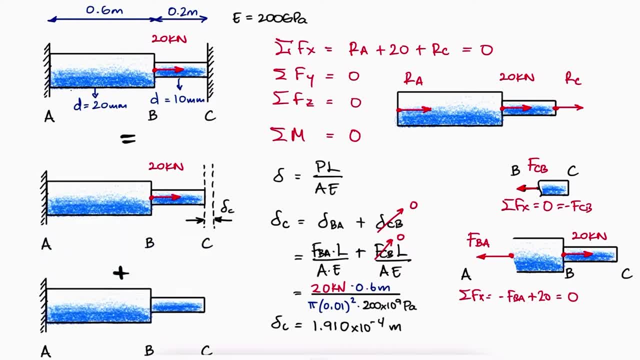 Then we would superpose a second scenario where the wall is now there at C causing a reaction, And because we already took care of the external load, this new superposed scenario doesn't have it in it. The quote-unquote trick here is that since 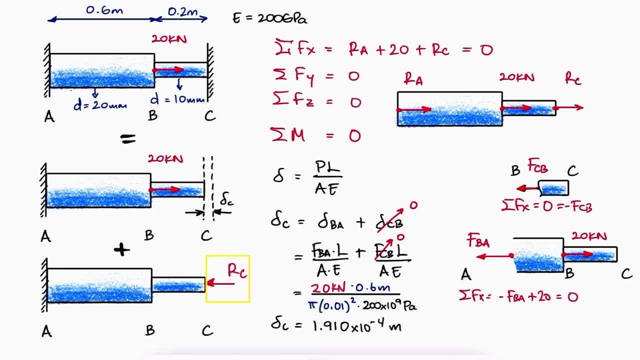 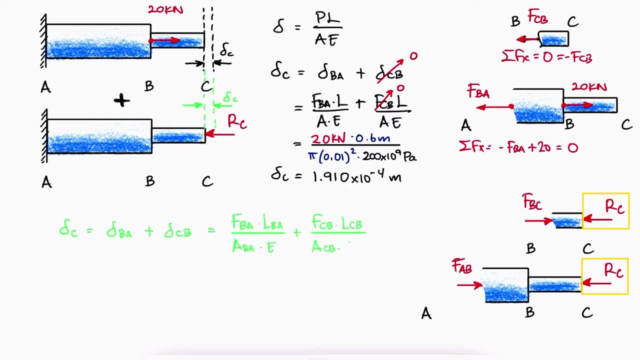 C is not moving. in the real scenario, the reaction force C in the second superposed case should be compressing the rod by the same amount that case 1 elongated it. Since the internal force in this second case is the reaction force at C, both sections are subjected to that force. 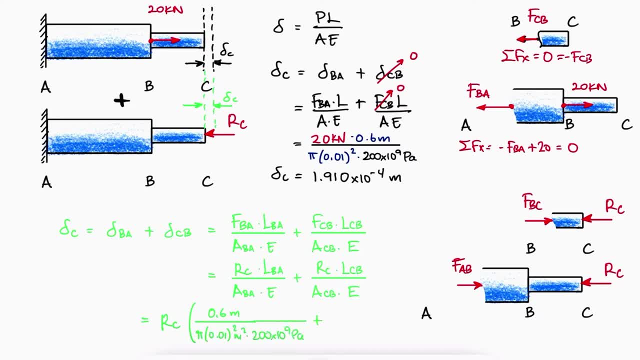 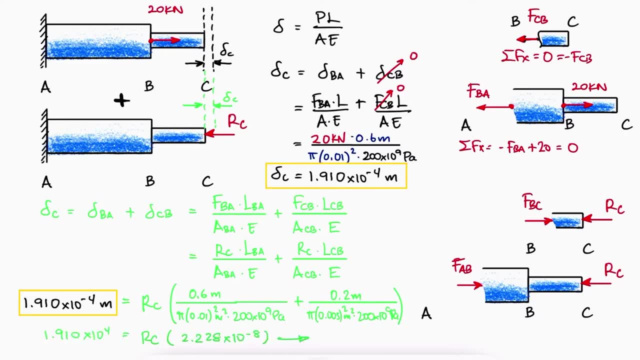 which means we can write two section deformation expressions with that being the internal load. By doing this we can solve for it using the information deflection. from the first case, With the reaction force at C, we can go back to the statics equation and solve for the reaction at A. 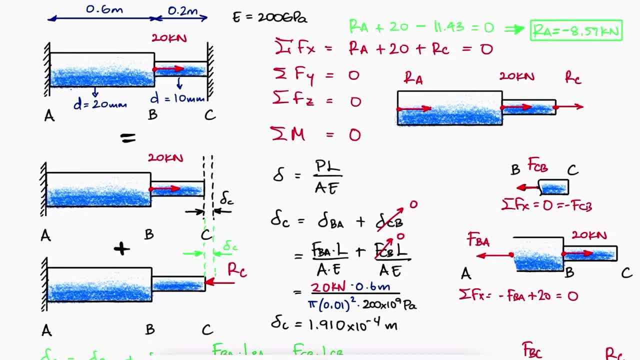 Like I mentioned before, this is only useful to you if your class instructor requires you to use the superposition method. We'll get back to it soon. So on the left-hand side of the slide we will see a copy of a very complex for-ел�� equation and also further details about how tovid 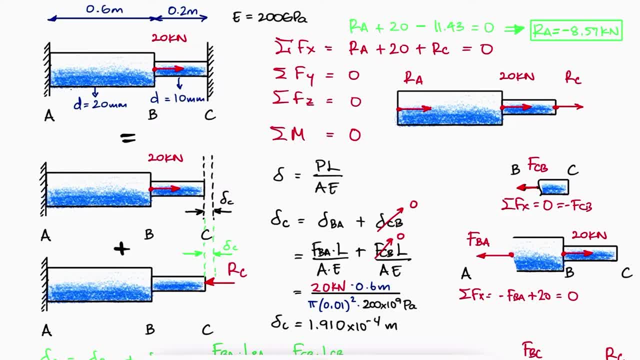 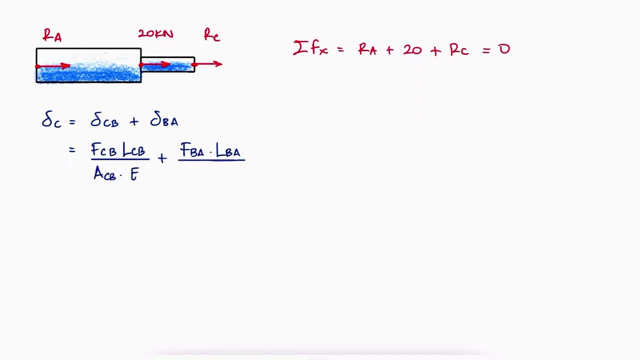 The main alternative- and it will always be a quicker procedure- is to just write the displacement of C in terms of the actual internal forces and equal that to its displacement of zero With the free body diagram, and always assuming positive reaction and internal forces which. 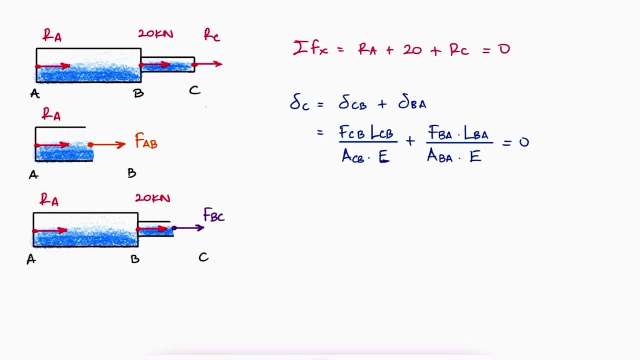 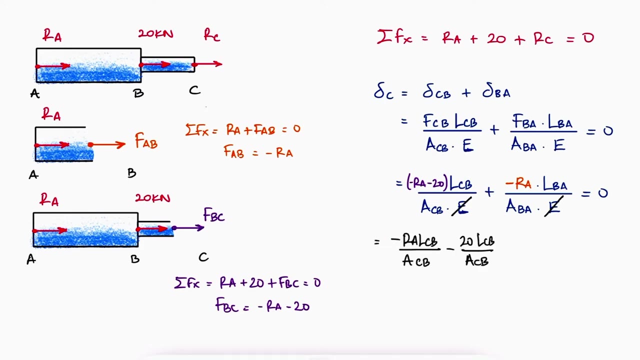 follows the very important suggestion and explanation covered in the previous lecture. we see that the internal force from A to B is minus R A and from B to C minus R A, minus 20.. Solving for R A and substituting the given values, we find the numerical solution for. 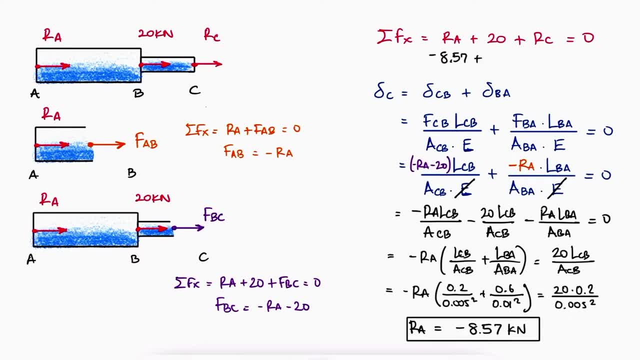 the reaction force at A and with that information and the sum of forces we solve for R- C. As you can see, without the superposition method we are not performing extra calculations like in this case. the theoretical decision, We have the displacement of C if the wall wasn't there, and we're not splitting. 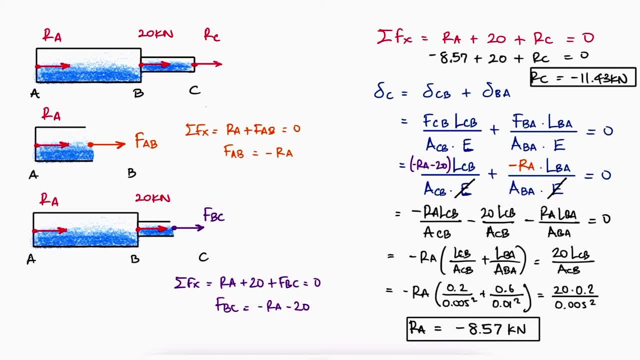 the problem into two axial deformation problems. We're only writing one equation that allows us to solve for one of the reaction forces right away. The negative values are of course expected, since the reaction forces would be actually pointing left. The reason we don't just assume the correct and very clear direction of the reaction forces: 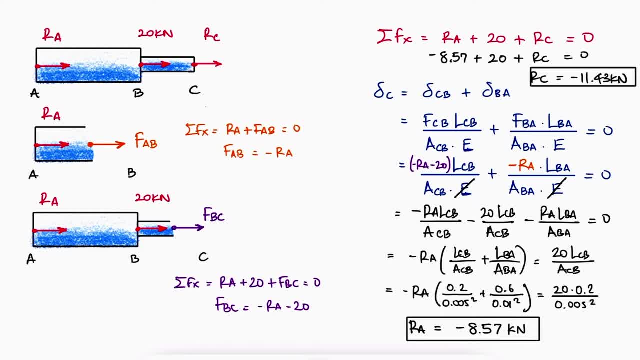 is precisely because of that It's not always obviously clear. The same happens with internal loads. We assume they are tensile. so if we get positive values, they are indeed tensile and for a negative value they are compressive, which follows the general convention for tension. 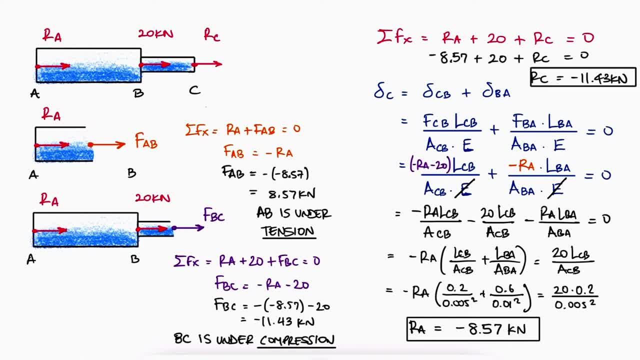 and compression. This is apparently clear when we substitute the actual values of the reaction forces in the free body diagram. AB is under tension and BC is under compression. Like mentioned before, statically indeterminate problems are also present in other types of stresses. 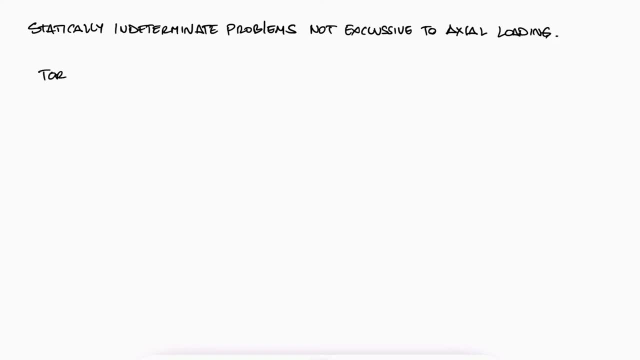 For example, torsion. An equivalent problem in torsion to this example would be to have an external torque applied to a rod within two walls. Statics alone would also give us one equation with two unknowns and we would have to use 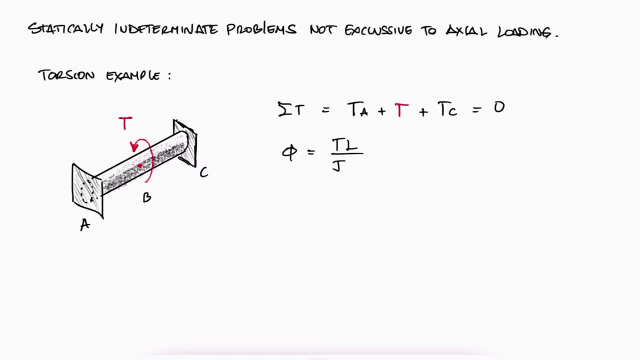 the deformation expressions, in that case the angle of twist to solve for the reaction torques at the walls. But more on torsion and bending, statically indeterminate problems. later Links below, Specifically for axial loading. statically indeterminate problems are also present in. 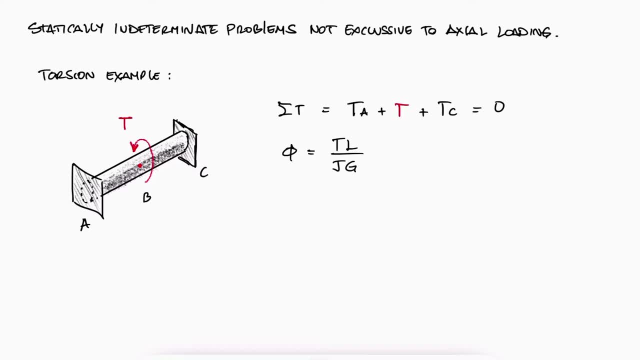 torsion. These problems can occur when other topics we've covered so far are also present, Like, for example, thermal expansion due to changes in temperature. that we already covered in the previous lecture video Link below. So let's look at an example related to temperature changes and keep in mind that the two scenarios 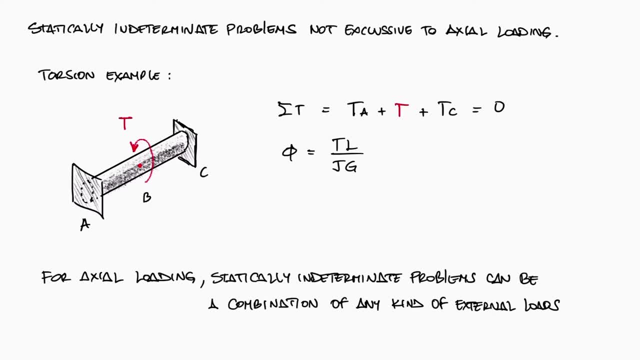 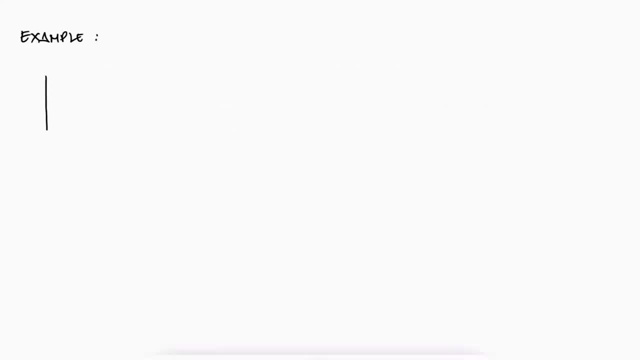 covered in this video are not the only types of statically indeterminate problems. For other examples, make sure to check the additional example videos linked in the description below. Let's look at a rod of two cylindrical rods. Let's look at a rod of two cylindrical rods. They are located in torsion of the wall on the sides. for example, as shown here, They are located in torsion of the wall on the sides of the board. So the δ-soul is located more in torsion of the wall and therefore have a further. 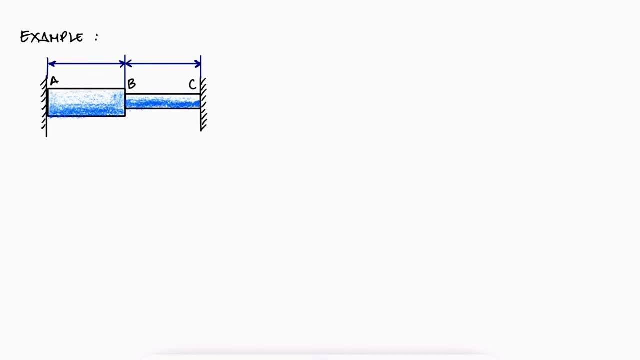 aspect of torsion. Let's look at a rod of two cylindrical rods. This is very similar to the rod of two vales, but they are not in torsion of the wall. This is the activation of the rod of two vales. 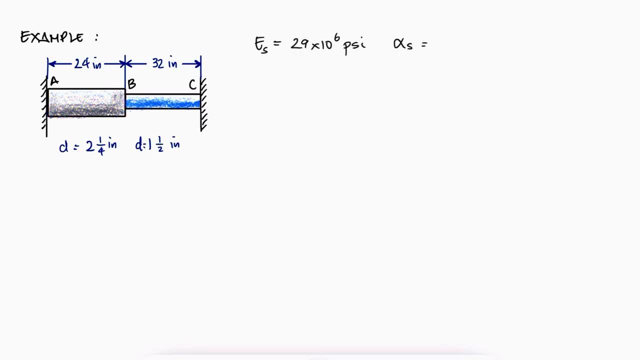 So, by the way, we have two holes. Here we are: the reaction forces of our rod and the reaction forces of our rod. The initial reaction forces are zero. By the way, that just means that the initial reaction forces at the wall are zero. 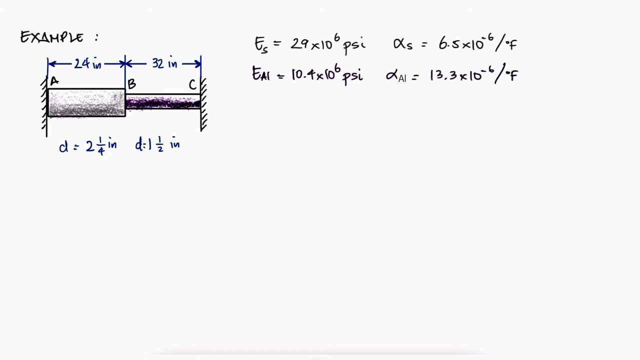 The ab portion is made of steel and the portion bc is made of aluminum. are the stresses in each section and what is the deflection of point B when there is a rise in temperature of 70 degrees Fahrenheit? Remember to try this problem on your own before. 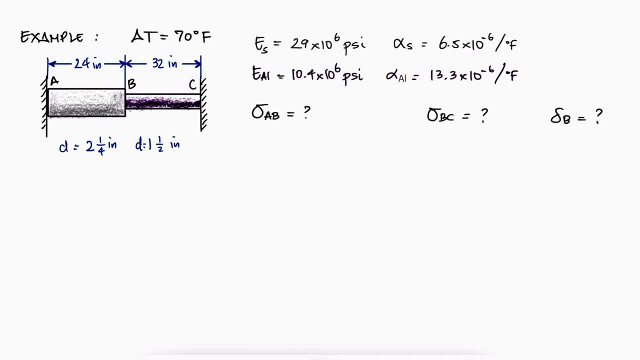 watching the solution. If the temperature rises, the member will try to expand, but since the walls won't allow that, the length of the member remains the same, even though the temperature change is trying to make it elongate, Finding the non-zero reaction forces at the 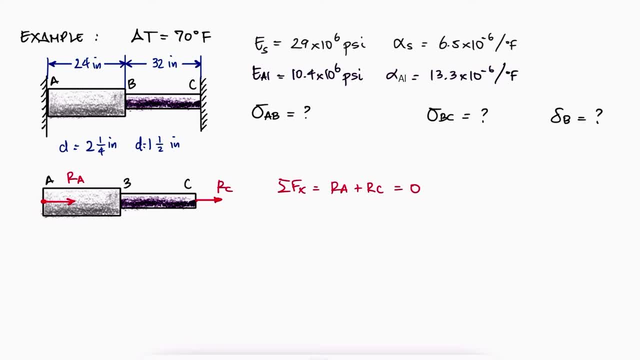 walls would be a statically indeterminate problem, since the statics alone would only show us that the reaction at C is the opposite of the reaction at A. However, we know that the deflection of A or C, whatever we want to use, is zero, So let's write that the 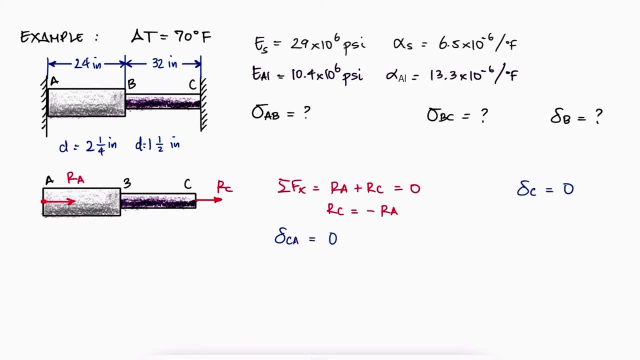 deflection of C with respect to A is zero, which means that the deflection of B with respect to A plus the deflection of C with respect to B is zero. From A to B, we have both an axial deformation due to the rise in temperature of C and a rise in temperature.